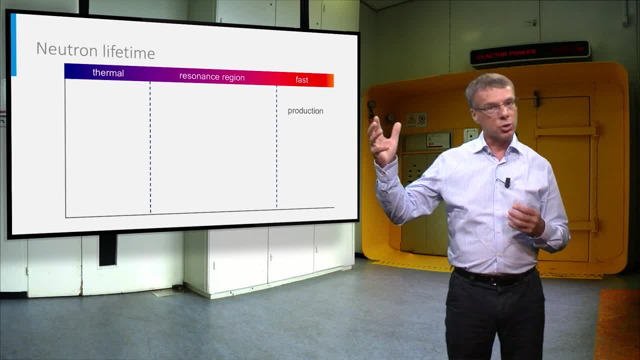 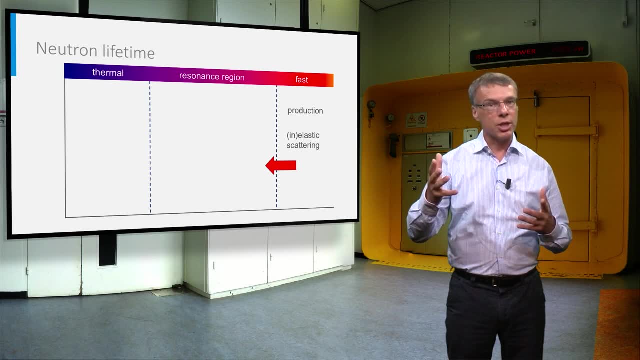 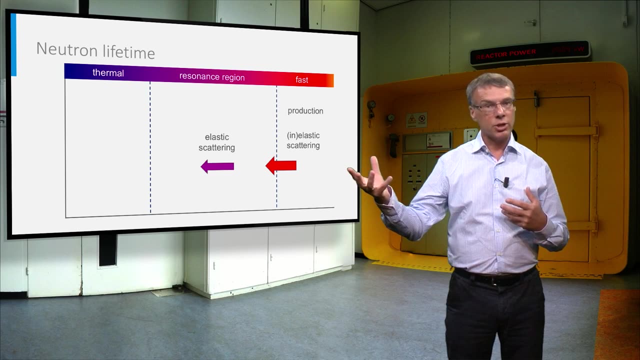 A fission neutron is released at very high energy of about 2 megaelectron volt And by elastic and inelastic collisions it will lose energy and reach the resonance value range of the uranium-238.. Here the neutron can lose energy via elastic collisions with the moderator, or it can be. 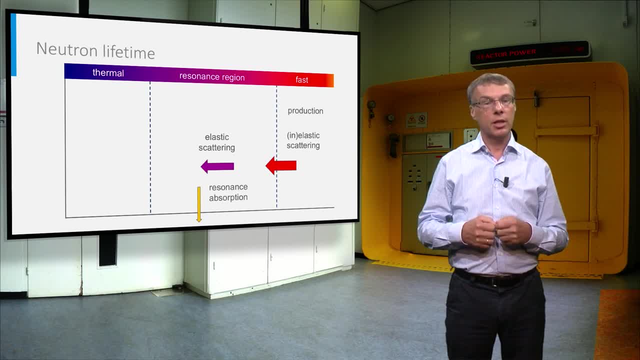 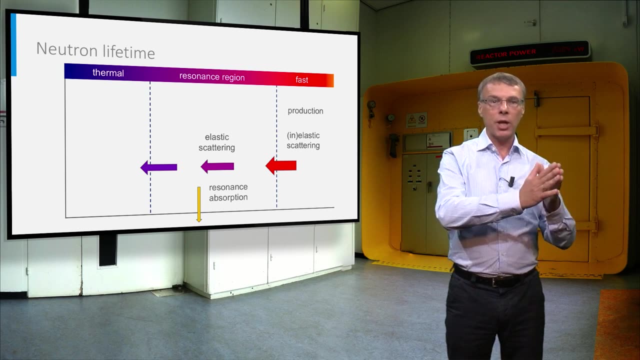 absorbed in the uranium-238 resonances. In the latter case, the neutron is lost for the chain reaction. Of course, this is also the case when a neutron leaks away from the reactor core. When the neutron survives the resonance range, it will reach the thermal energy range and 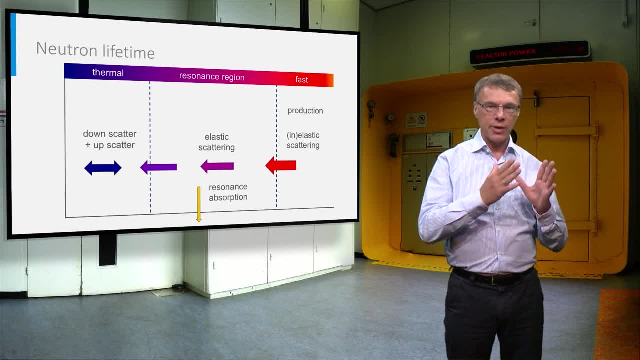 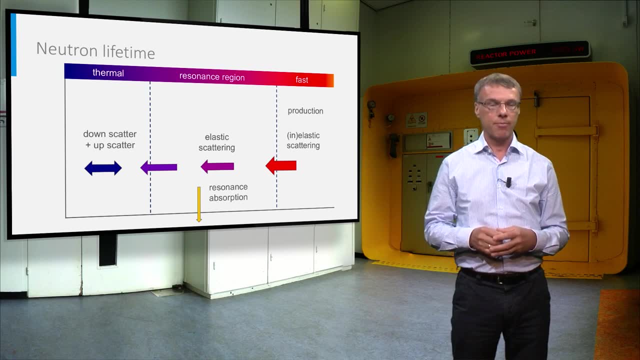 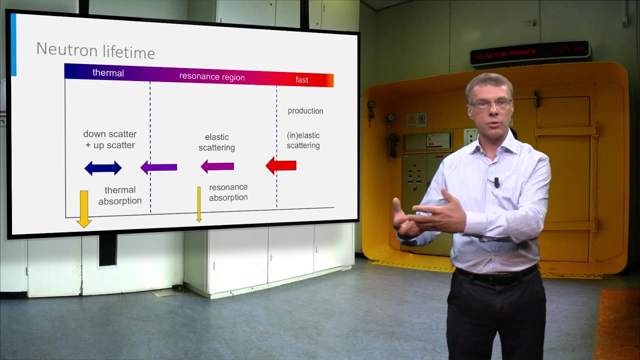 this range is very special Because the moderator atoms have an energy comparable to that of the neutrons, which means a neutron can also gain energy in a collision. But eventually all thermal neutrons will be lost via absorption in the reactor core or via leakage out of the core. We will now follow the fission neutrons in more detail between birth and death. When the neutrons are released at high energy, some of them will be absorbed by uranium-235 and uranium-238.. And, although the chance is not very high, some of these absorption processes can lead. 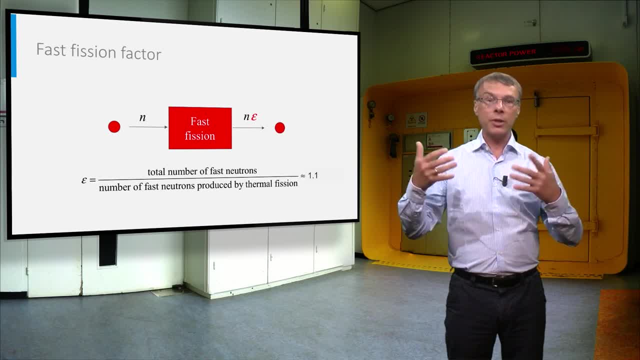 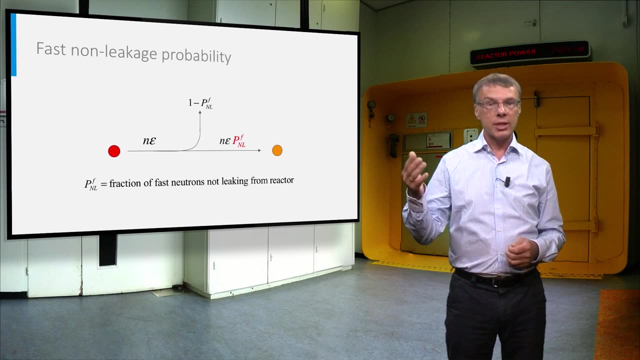 to fission of uranium. In this case, we will gain some neutrons, And if we start with n neutrons, this number will be multiplied by the fast fission factor, epsilon, which has a typical value of around 1.1.. When the neutrons still have a high energy, they can escape from the reactor core. 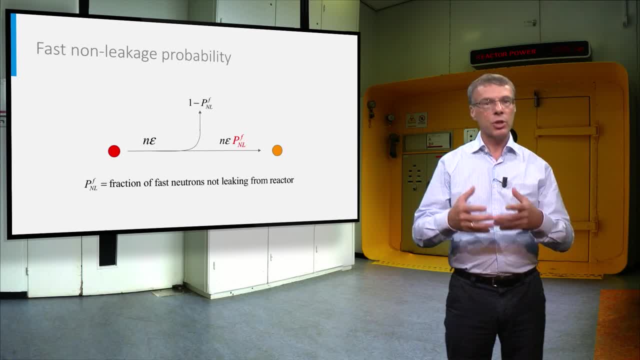 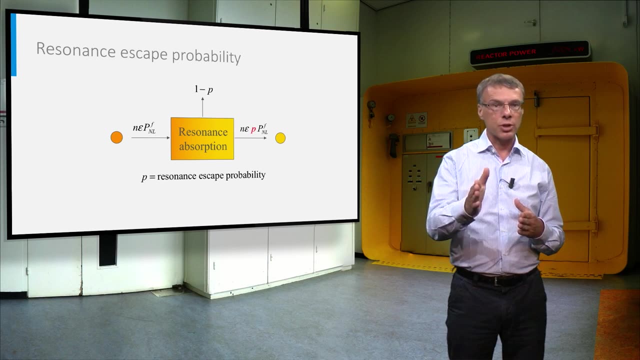 The fraction of neutrons that survives leakage is called the non leakage probability, And because we speak here about fast neutrons, this fraction is called the fast non leakage probability. As mentioned before, the neutrons that slow down have to cross the resonance region of 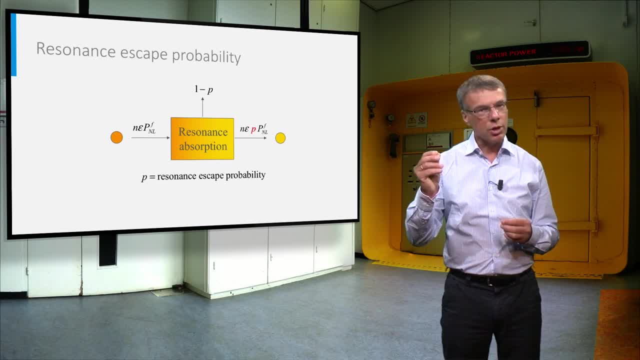 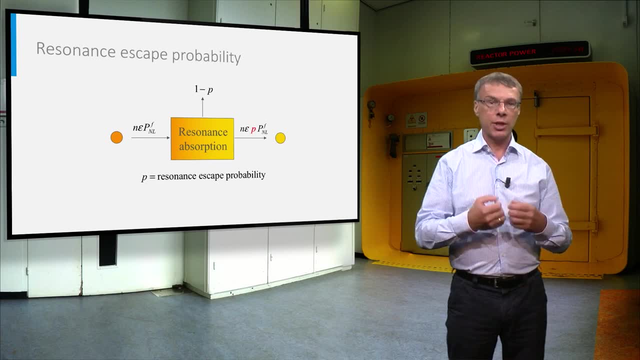 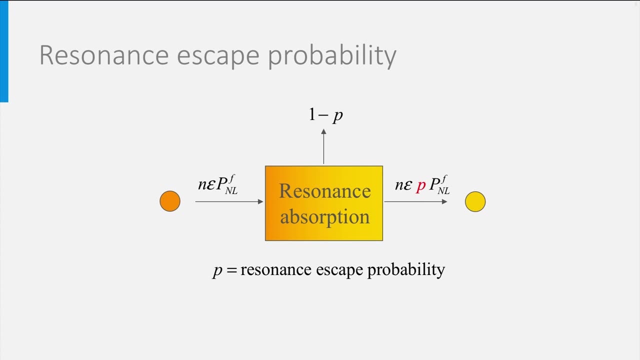 the uranium-238 in the fuel. A certain fraction of the neutrons will be captured, while a fraction, p, called the resonance escape probability, will survive the resonance range. resonance range: The number of neutrons indicated on the right hand side of the square- have survived the 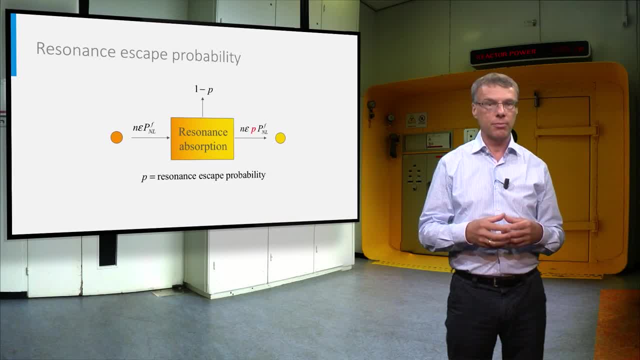 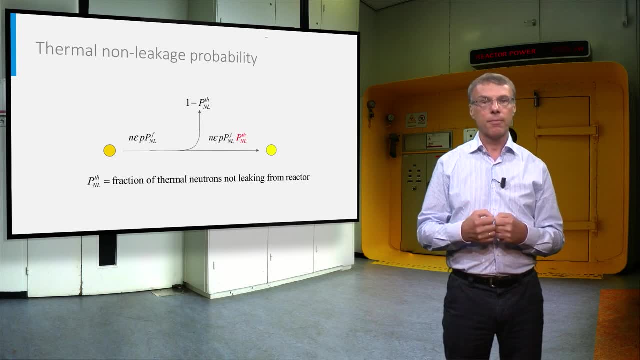 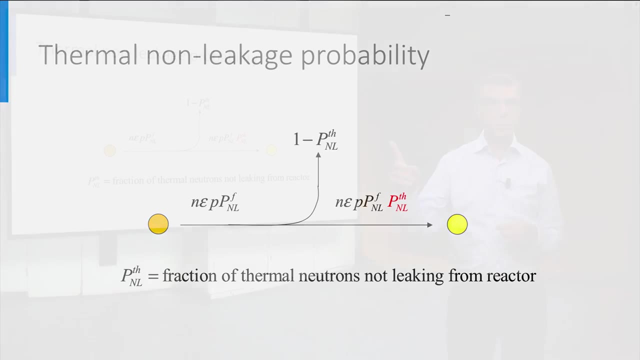 resonances and will reach the thermal energy range. The thermal neutrons can disappear from the reactor core either by leakage or by absorption. The fraction that survives leakage is called the thermal non-leakage probability, indicated with the red capital P in the formula.